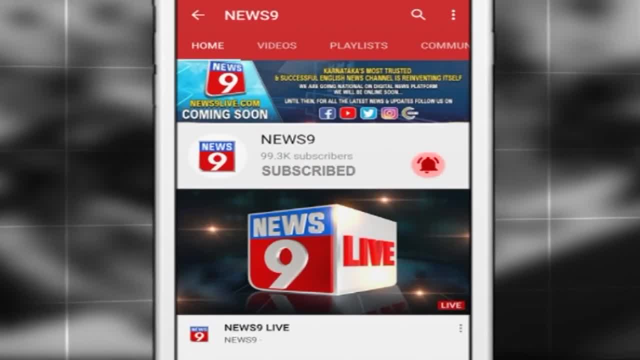 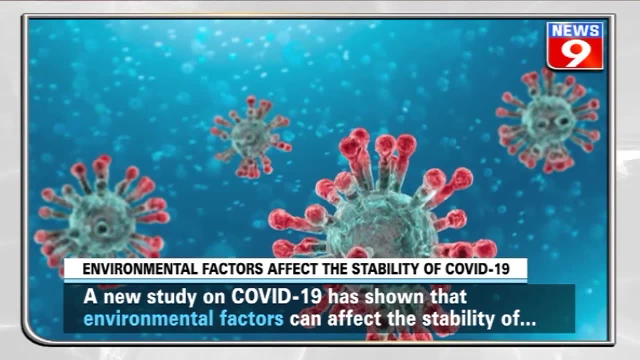 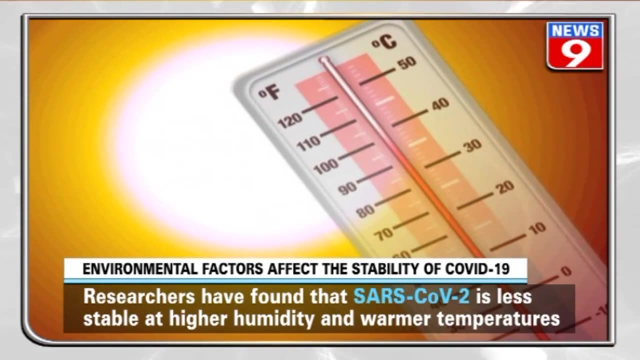 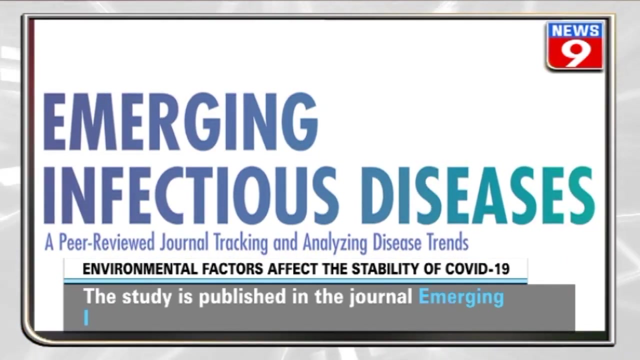 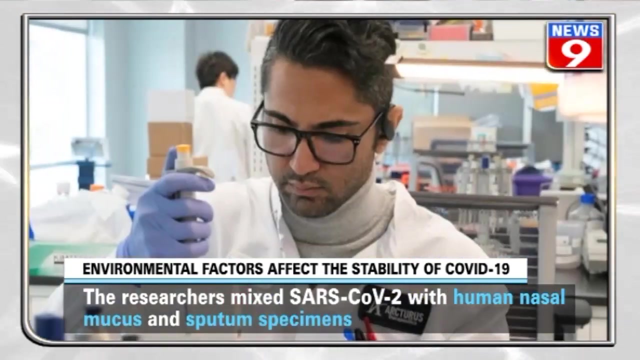 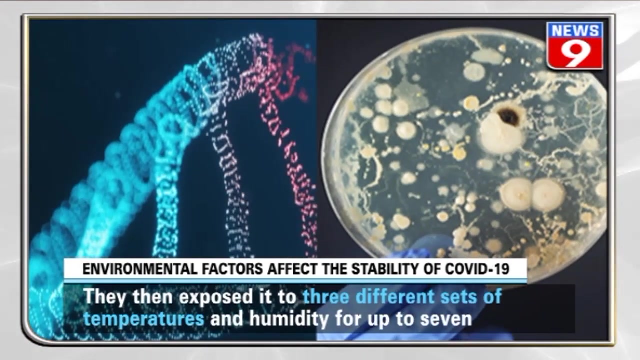 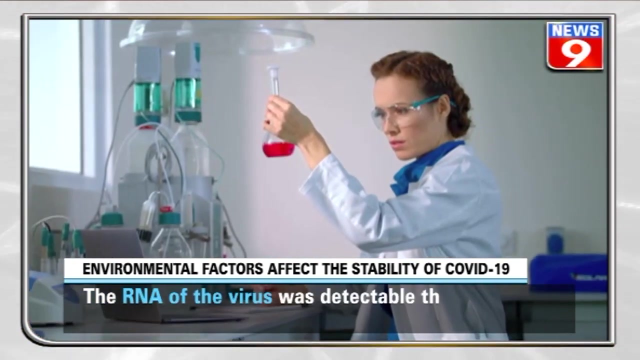 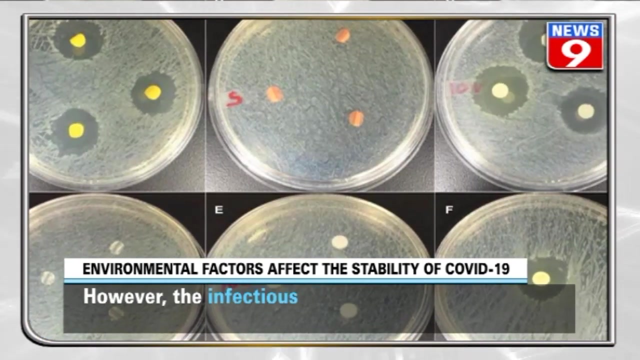 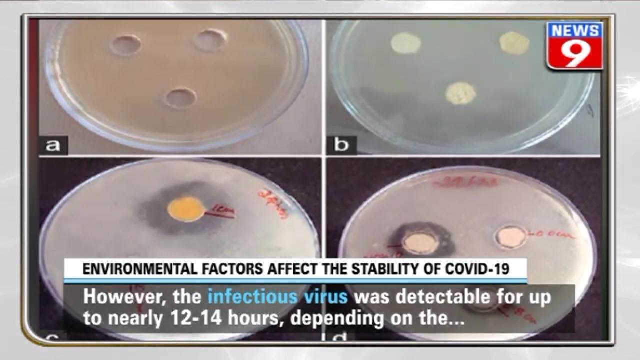 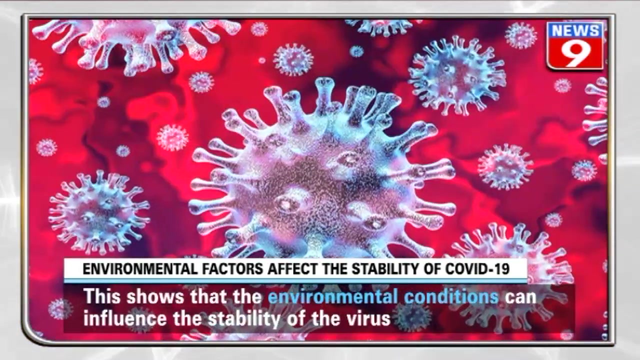 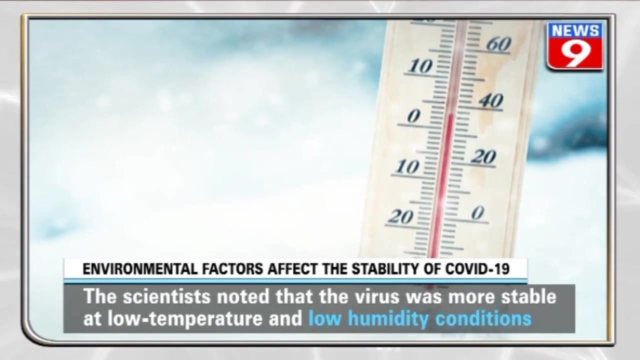 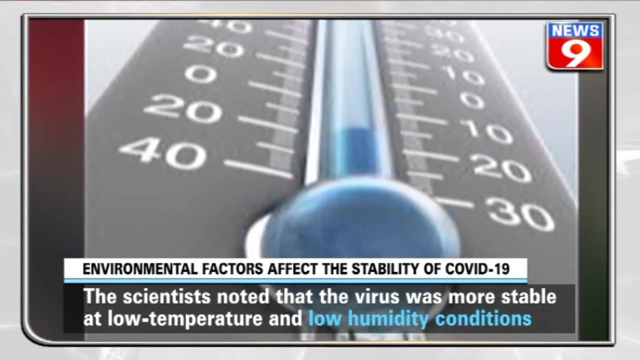 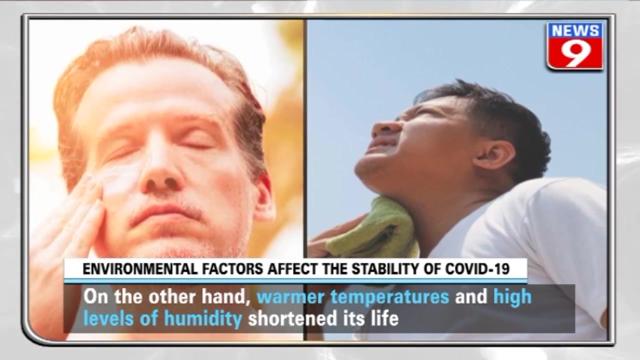 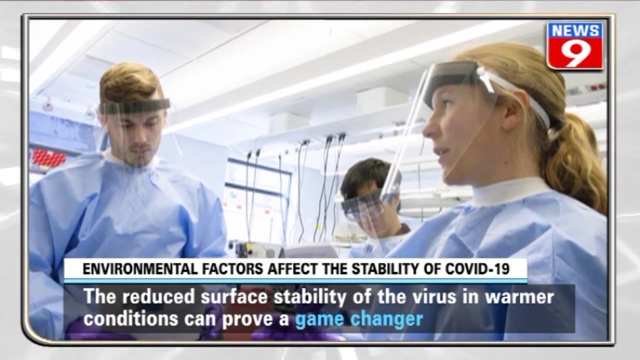 For all the latest updates, subscribe to News 9.. For all the latest updates, subscribe to News 9.. For all the latest updates, subscribe to News 9.. The reduced surface stability of the virus in warmer conditions can prove a game-changer. 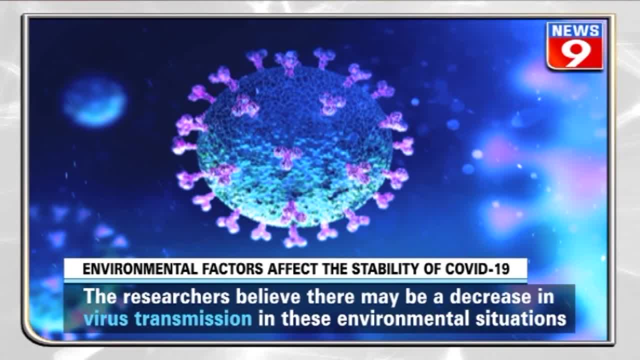 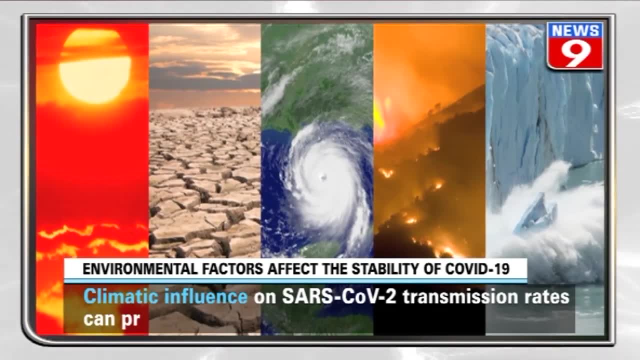 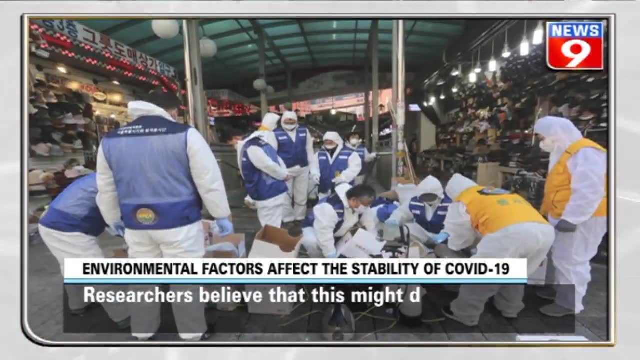 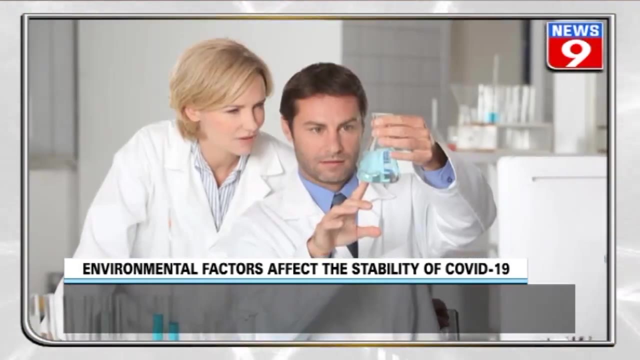 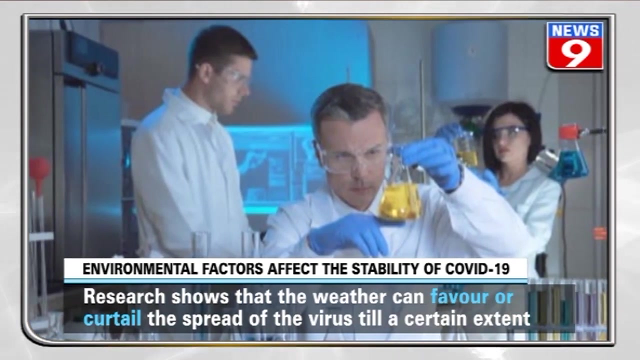 The researchers believe there may be a decrease in virus transmission in these environmental situations. Climatic influence on SARS-CoV-2 transmission rates can prove costly. Researchers believe that this might drive seasonal outbreak dynamics in the post-COVID era. Research shows that the weather can favor or curtail the spread of the virus till a certain extent. 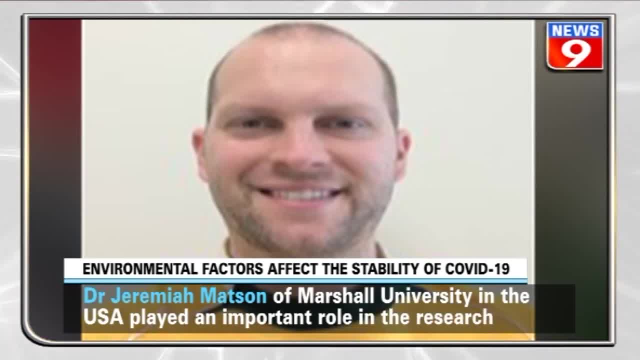 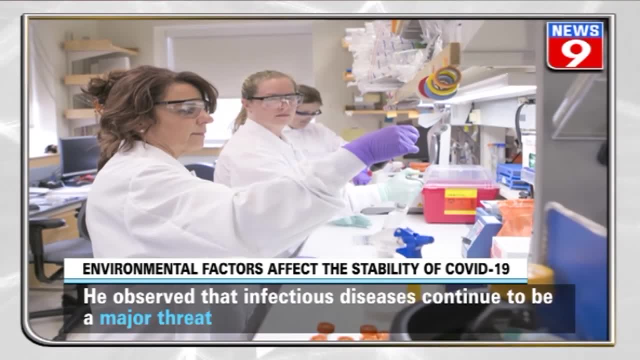 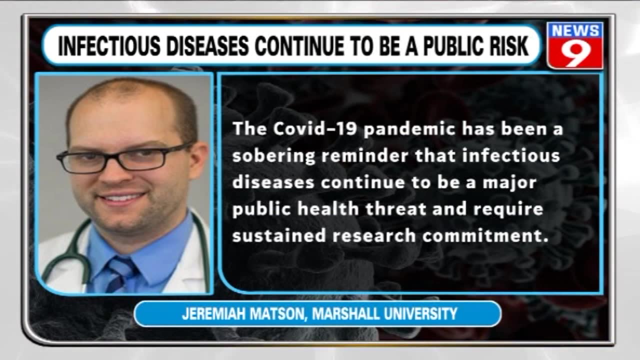 Dr Jeremiah Madison of Marshall University in the USA played an important role in the research. He observed that infectious diseases continue to be a major threat. The COVID-19 pandemic has been a sobering reminder. An infectious disease is a known trial. The COVID-19 pandemic is known for many members of the public citizens: P malt, an infection. that infection diseases continue to be a major public health threat and require sustained research commitment. 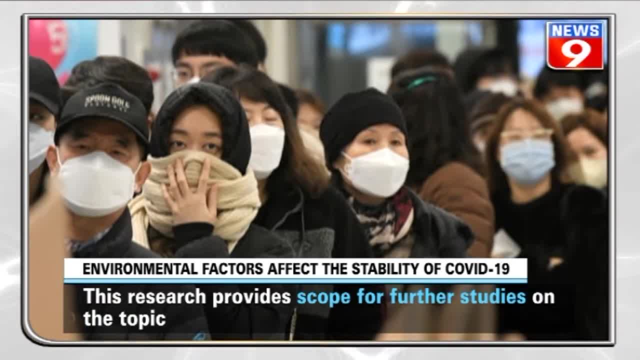 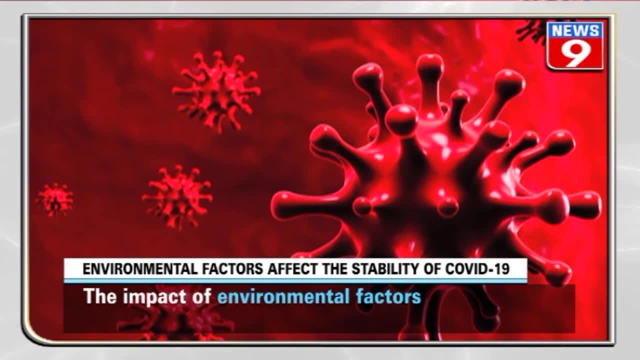 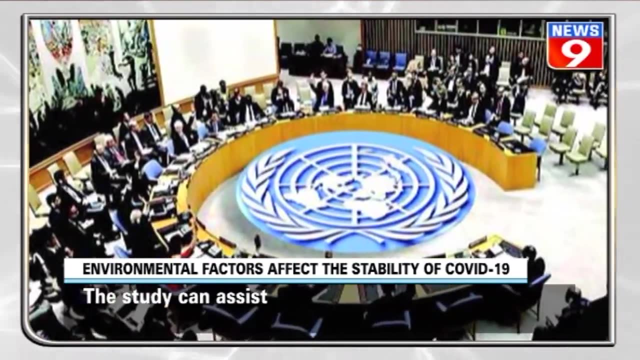 This research provides scope for further studies on the topic. — Tim Ionga. purchaser contact info. The impact of environmental factors on the virus can make it stronger in certain conditions. The study can assist policy-makers to take the required protective measures. Du Bthinking Involves Breaking Cases of the COVID-19 Problem.